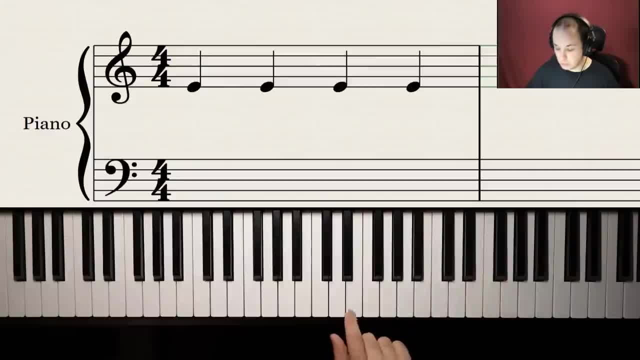 So a tempo just tells you how fast you play. A fast tempo: one, two, three, four. one, two, three, four is counted and played very quickly. A slow tempo: one, two, three, four is played slow. 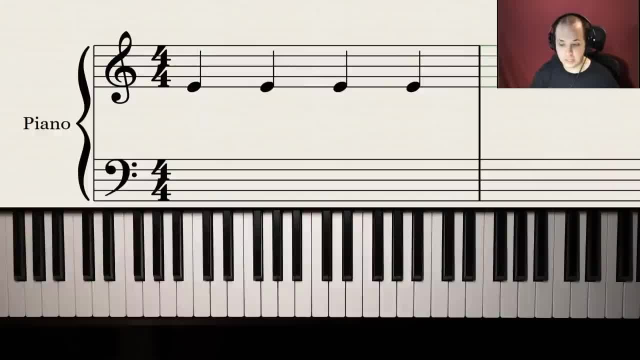 And tempo is usually expressed as a number. It'll say like quarter note equals 120 in the beginning of the song, Or they'll use it as like an Italian word. So if it says adagio, that means you're going to be playing with a slow tempo. 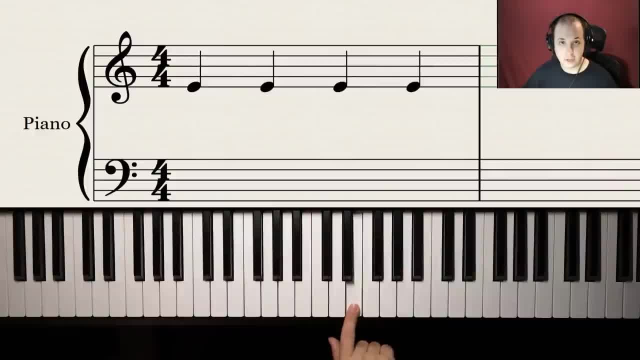 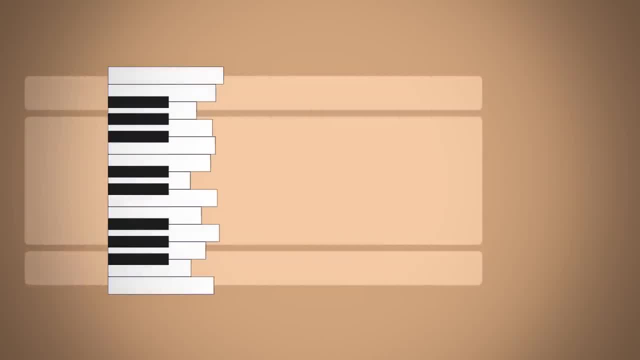 One, two, three, four. So that's all there is to tempo. Let's move on to the next topic. Now we're gonna talk about note durations. A note duration, very simply, is how long you're gonna be playing the note for. 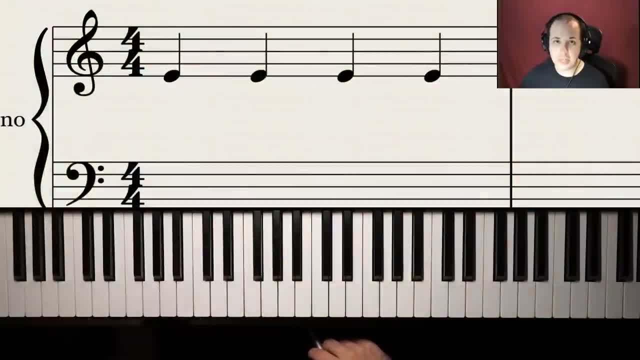 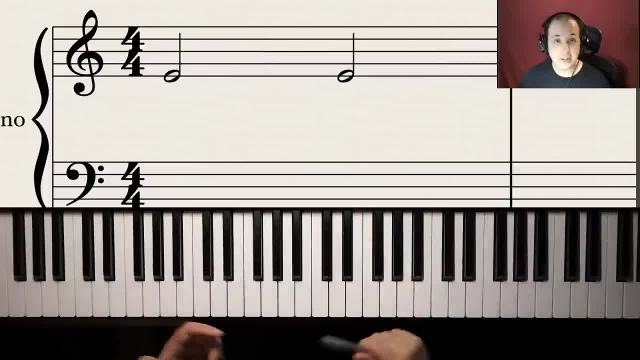 So let me give you a few examples of these. So here I have two half notes right now. How many beats does a half note get? Well, it gets two beats right, Assuming that you know all of your note durations. you know quarter note gets one beat. 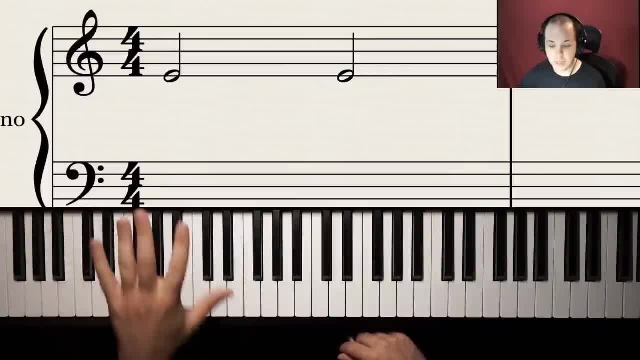 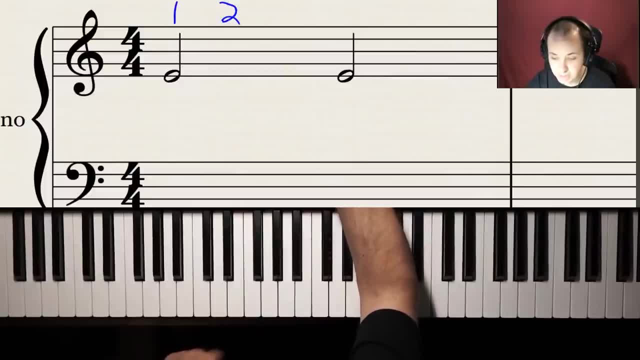 half note gets two, dotted half gets three, whole note gets four. So here we have two half beats, We still have, or two half notes, rather we still have four beats in the measure right. So you have two beats there, you know. 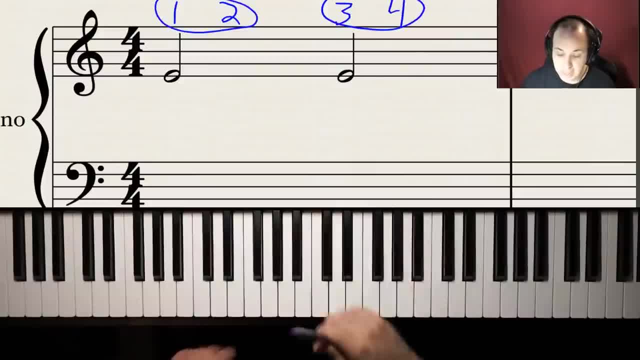 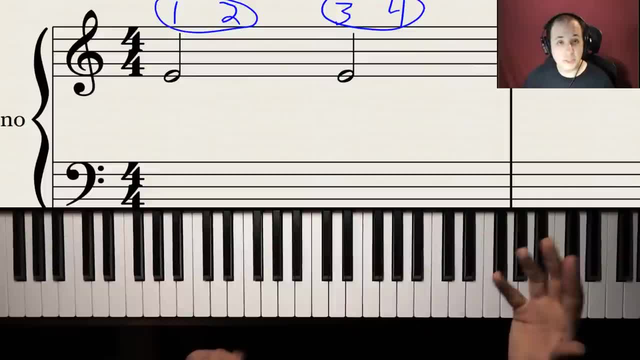 and two more beats. there beats three and four. We'll talk more about how to count these in a minute when we talk about time signatures, But right here we have one, two, three, four. I'm still counting to four in this measure. we call it. 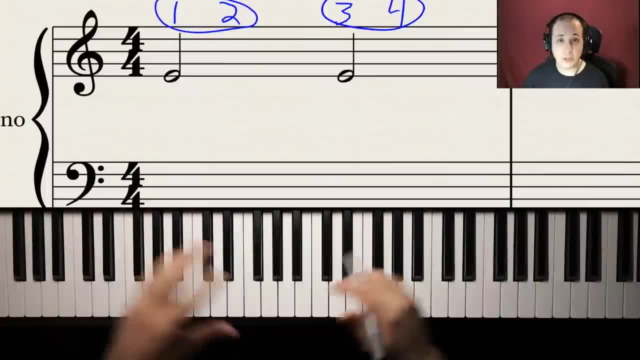 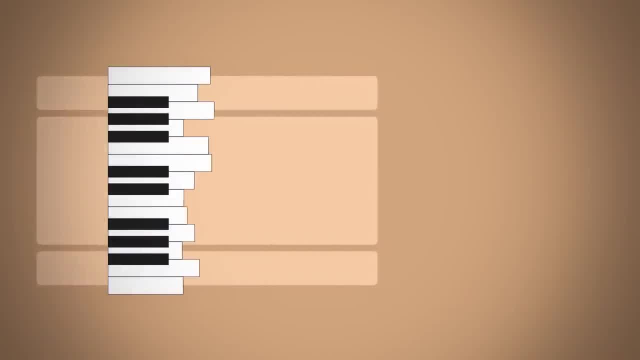 and we're just playing the notes a little bit longer, So those are called the note durations. They are the duration in which you hit the notes. Now we're gonna talk about measures, So if you notice that music is broken up by these verticals, 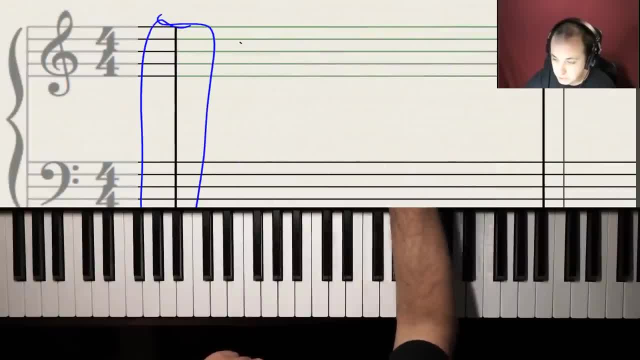 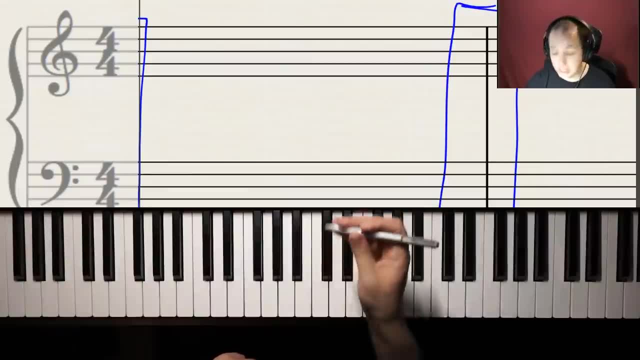 Vertical lines, right, Look right there, there's one, There's another one, let's find one more. So there's a third one, right, And those are called the measure lines, But they aren't really the measures themselves. they just kinda tell us where the measures take place. 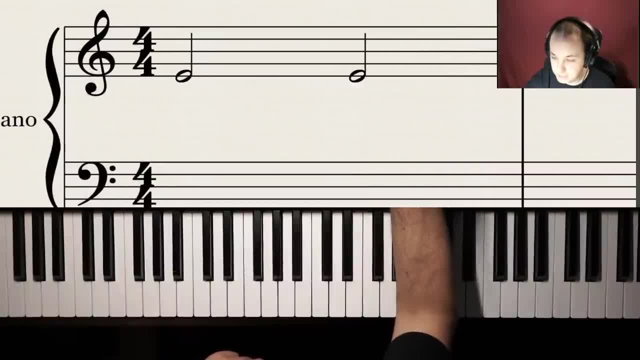 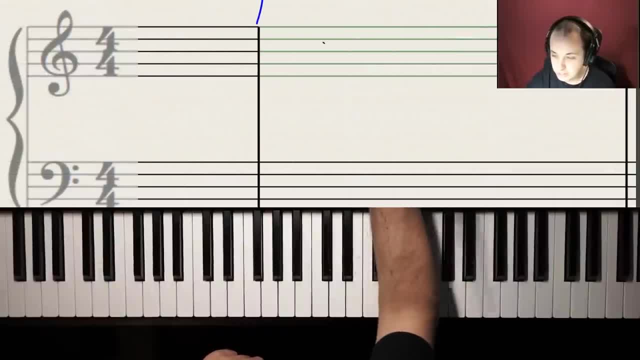 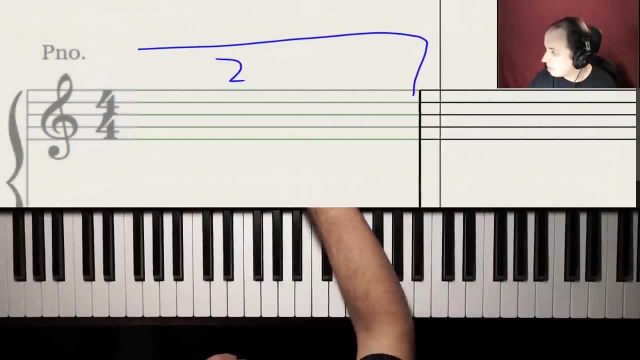 The measures themselves are the distance between. you know each of these boxes. So measure one is right here, Measure two is right there. Let me actually scroll that down for us. So you have measure one in that box, measure two right there. 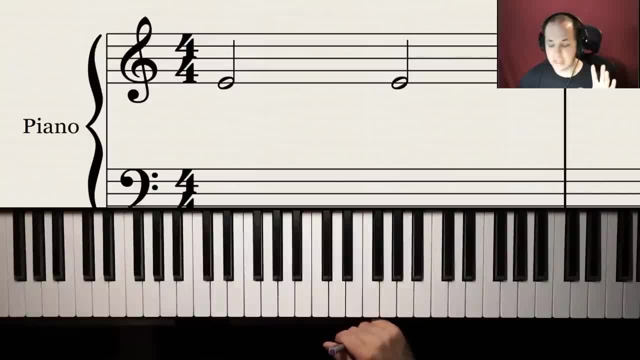 So what are measures for? Well, measures are really so we can break up the music and read it a little bit easier. It just helps really organize the music into little units, right, And they are based on the thing we're gonna talk about. 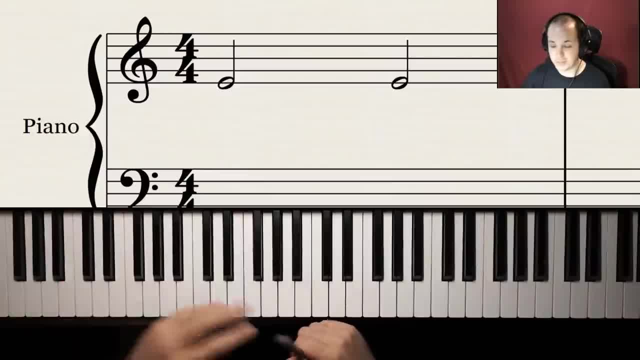 in a minute here called the time signature, which I'll tell you what that means in a second. But basically we're fitting so many beats into each of these boxes, right? So that's what we're doing, And it just really makes it a lot easier. 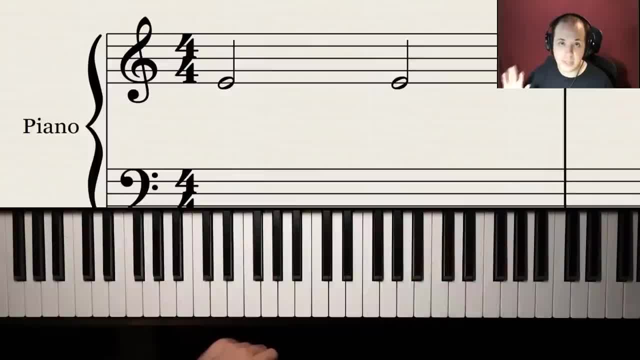 to follow the song. So if you're playing in a band and the instructor says, or the director says, play starting from measure 10, you'll know where that is, And usually there's what we call measure numbers at the top of the page. 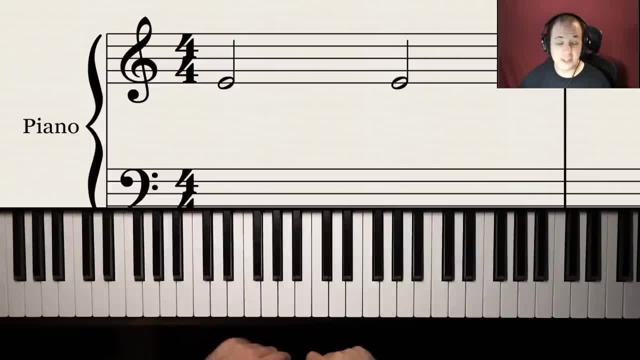 Not at the top of the page but like right above where the measure is, to tell you what number measure you're currently on. So that's all there is for measures. Just know that they are these little boxes that really help break up the music. 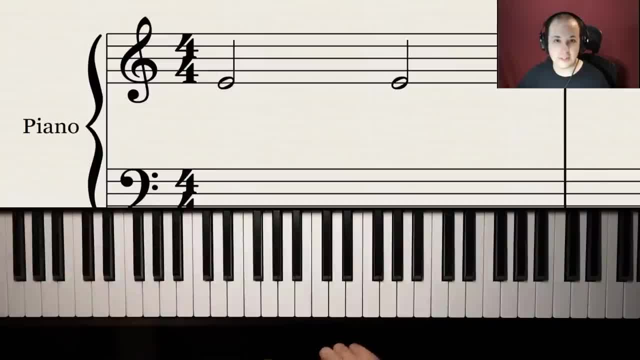 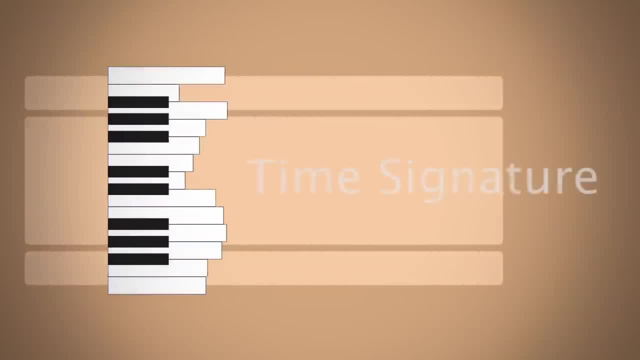 into more digestible and easier to understand smaller units. Now we're gonna talk about this thing called the time signature. So where is the time signature usually located? Well, it's usually located right at the beginning of the song. Let's pick a fancy color here. here's red. 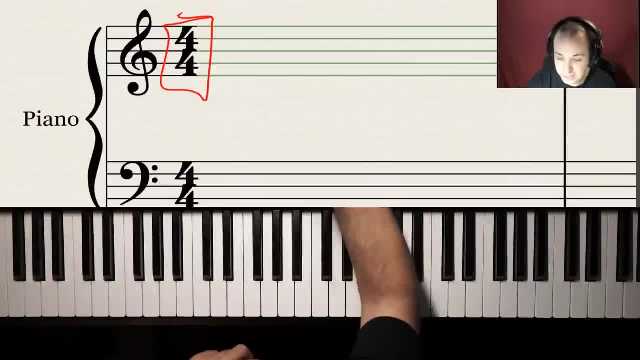 And that is not the time signature. Here is the time signature, right next to the clef. So right, and you say it by the first number, first on the top, so four, and then the bottom number, four, So that one is called four, four. 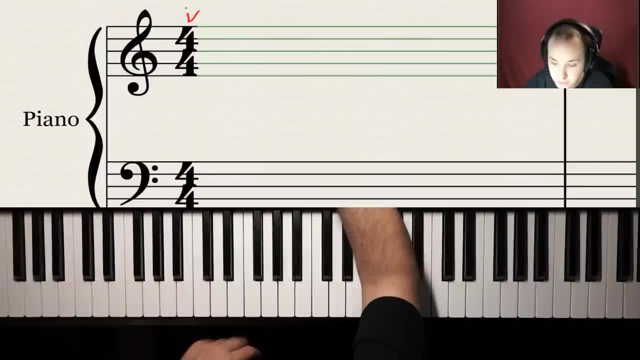 So that's the time signature, And what it tells you is: the top number tells you how many beats in a measure and the bottom number tells you which one gets one beat. So it ends in a four. so what note gets one beat? 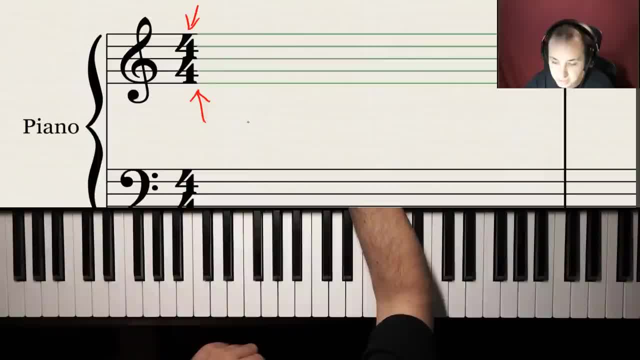 What does that tell us? Well, think about it this way. right, so it's four over four. Pretend for a minute like the top number is just a one, And that just makes it easier. So just pretend the top number's a one. 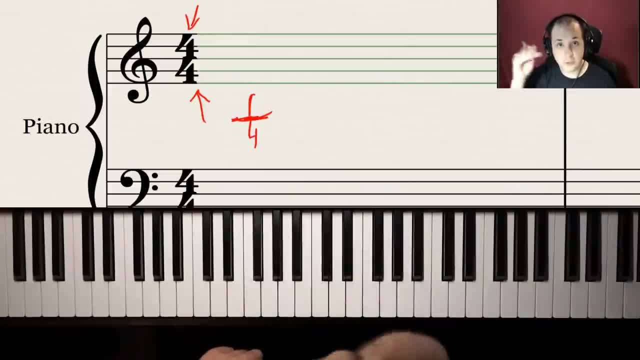 And then write the bottom number as it regular like. so you have one over four, right? Well, what is one over four, commonly called, Well, a quarter, right, Like? if you have a quarter of a pie, there is a quarter. 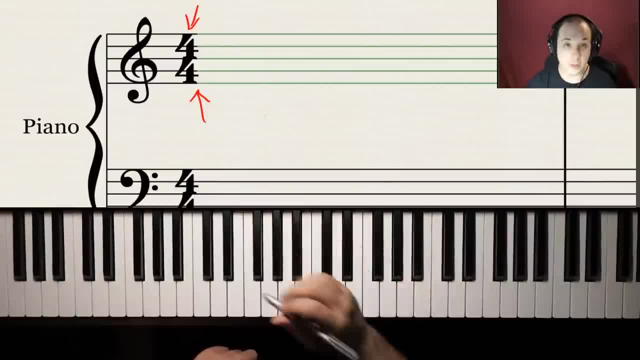 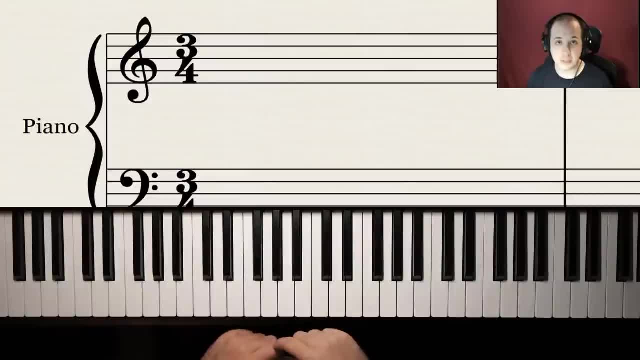 So that's telling us that the quarter note is going to get one beat. Now what happens if it says three, four? Let's choose that. So now it's three, four. well, what's changed? right, Only the top number. so we're only changing. 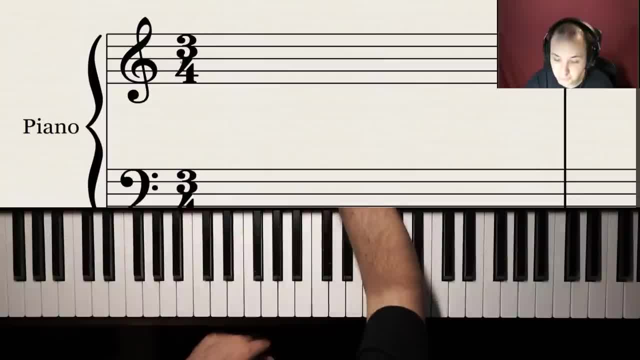 how many beats we can fit in this measure. The bottom number four, still remains the same, So a quarter note gets one beat. So a way I would think about this is that this is telling us that we have three quarter notes or equivalent to. I mean they could be eighth notes. 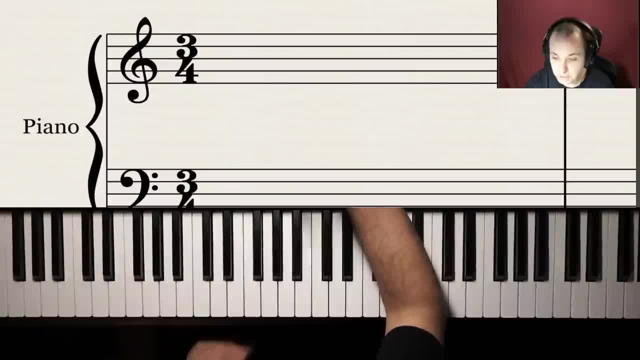 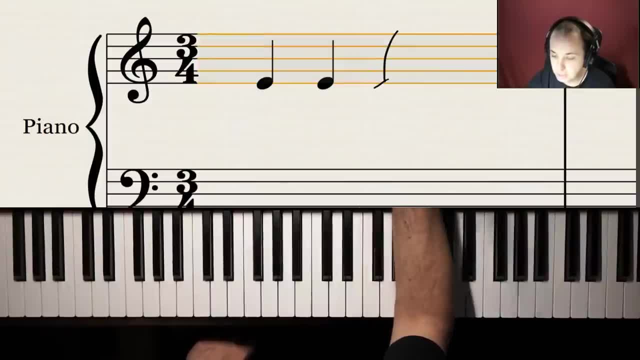 or whatever in each measure. So let me show you how to fill in just this measure as a quick example. So it's telling us right, we can have equivalent to three quarter notes in that measure, That's if it cooperates with us. 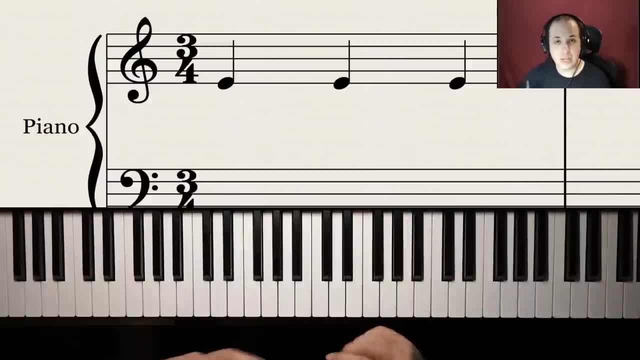 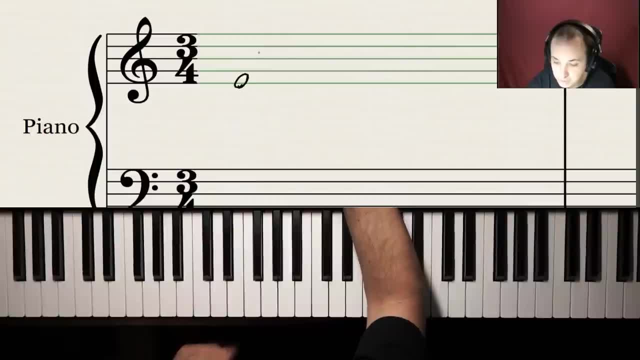 There we go, three quarter notes. You know we're not gonna talk about all the note durations today, but you could also fit, you know, a dotted half note which in itself would equal three. Now let me add a quarter note. 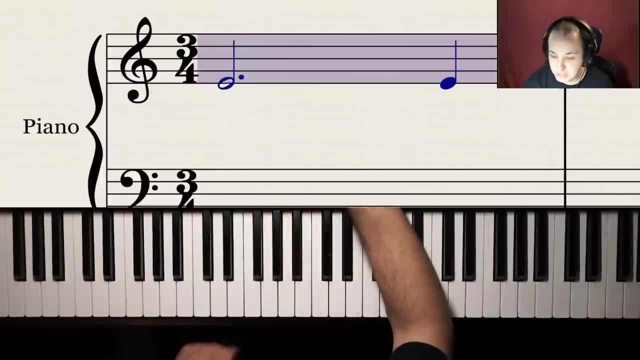 That is incorrect. Now, why is it? Well, it's because in this it actually kind of made it glow red a little bit, or highlighted it red, And that's because we have too many beats in that measure. So this measure has too many beats in it. 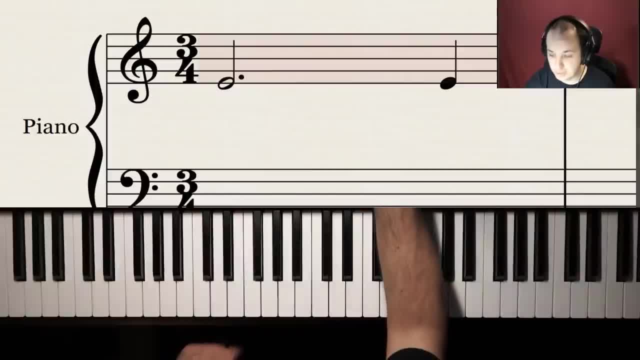 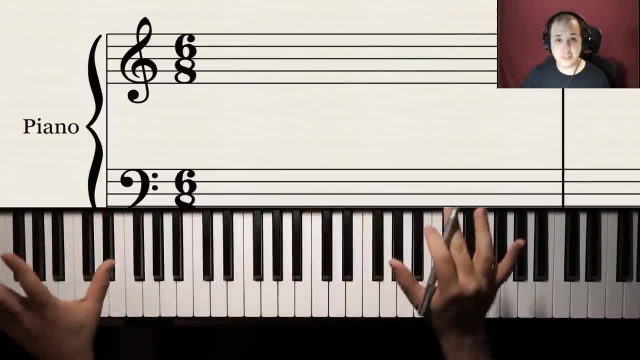 Now, if we were in four, four, that would be fine, since four beats would allow us to have four beats in that measure. Let's talk about one more time signature. So here we have six, eight. What's different about this time signature? 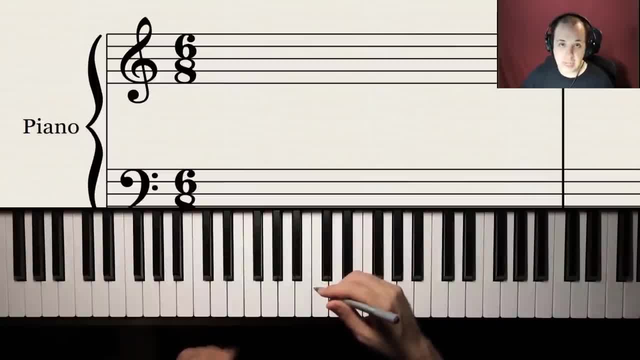 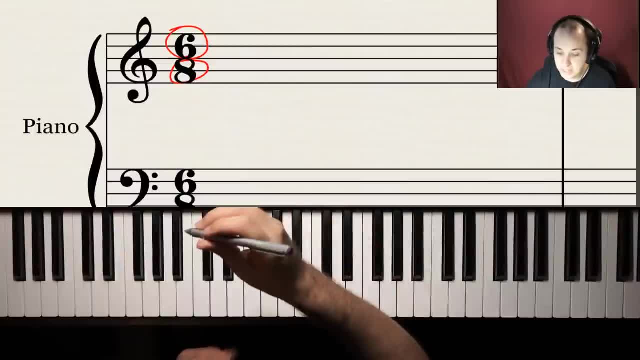 The top number is now a six right And the bottom number's now an eight. So what it's telling us? basically, remember that. it's telling us that there are equivalent to six eighth notes. in that measure. Now, what note gets one beat now? 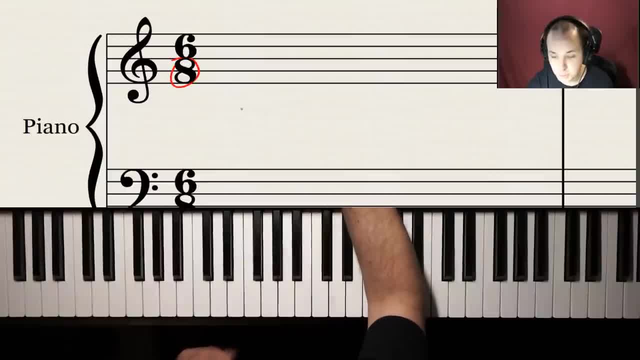 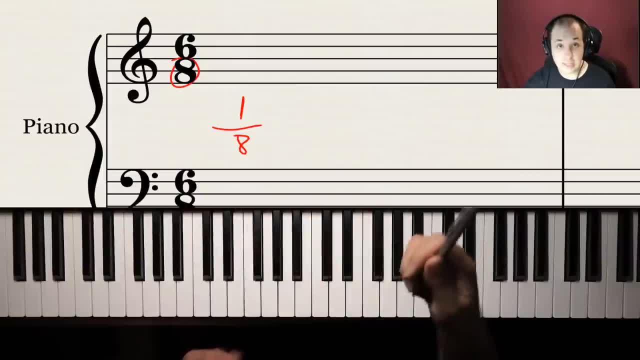 Well, it's the bottom number eight, right? So remember to figure this out. You just pretend like the top number's a one. You write the bottom number as usual, And hey, what fraction is that? That's one eighth, where the eighth note gets one beat. 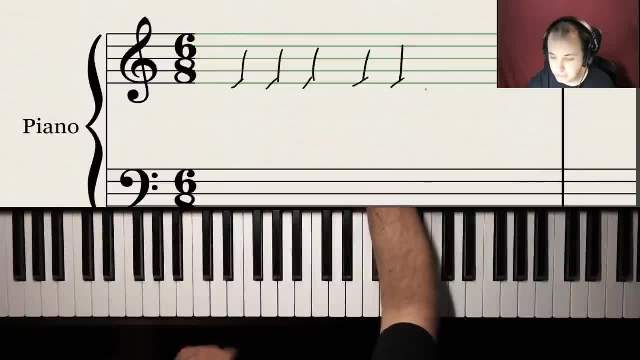 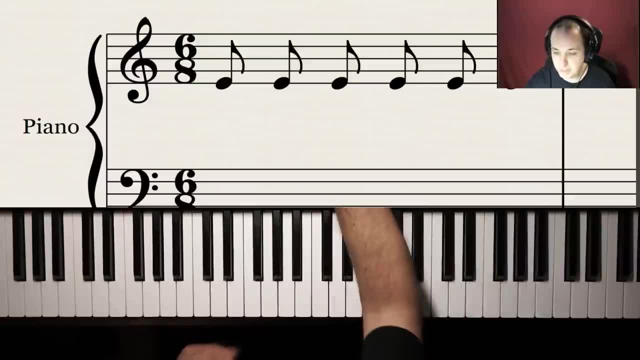 So now I'm gonna draw out a measure of six, eight, And these all need to be eighth notes. And there we go, they're six, eight Commonly. they kind of beam them across like that. But we have six, let's count them. 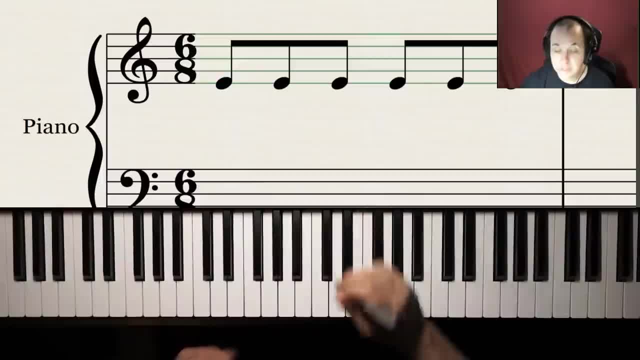 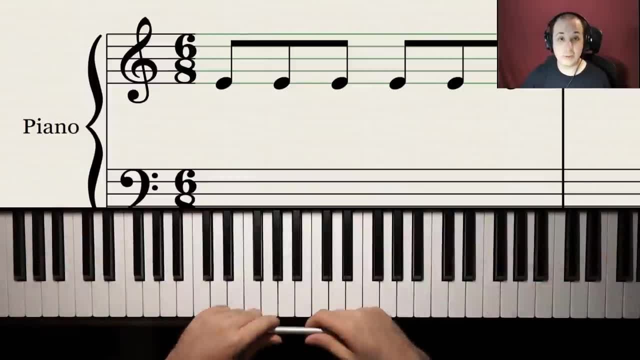 one, two, three, four, five, six, eighth notes in that measure. So let's move on to the final topic of today, which is defining exactly what rhythm is kind of tying everything together here. So how would I define rhythm, right? 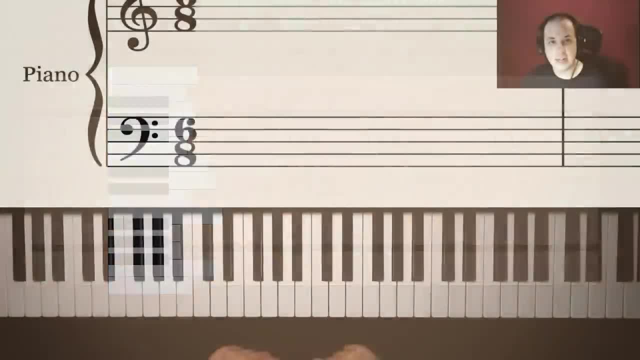 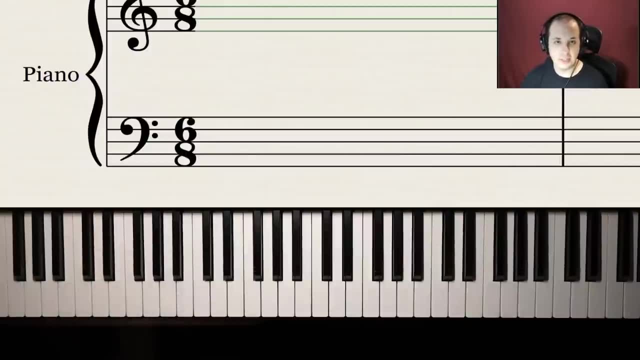 Well, I would define rhythm right. Well, I would define rhythm right As a combination of note durations and beats. It's really a recognizable pattern that you can find in a piece of music, which has to do with how long you're playing the notes. 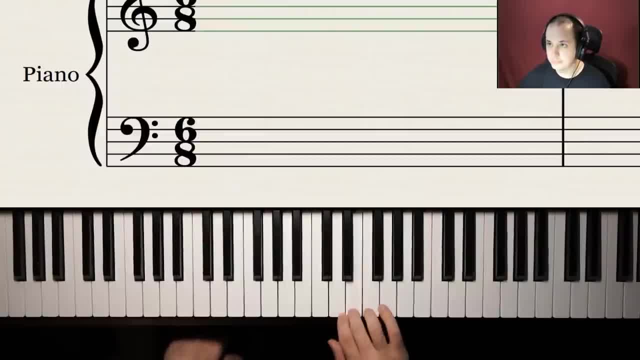 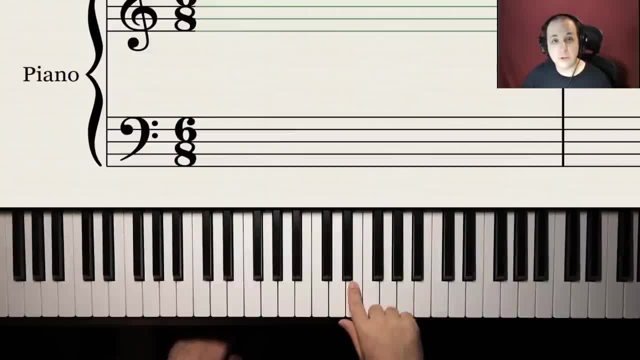 Or you know, just simply having four quarter notes, One, two, three, four, one, two, three, four- That's a rhythm too. It's a very simple rhythm, right? You're just playing the beats. So if you're just playing steady beats, 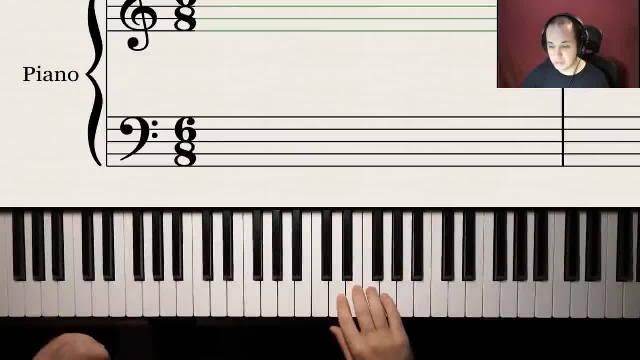 that can be a rhythm. But just because you're playing a rhythm Doesn't mean that all those notes are beats in themselves. They're all grouped together into beats. But just be careful that there's that discretionary thing. There's a little discrepancy there. 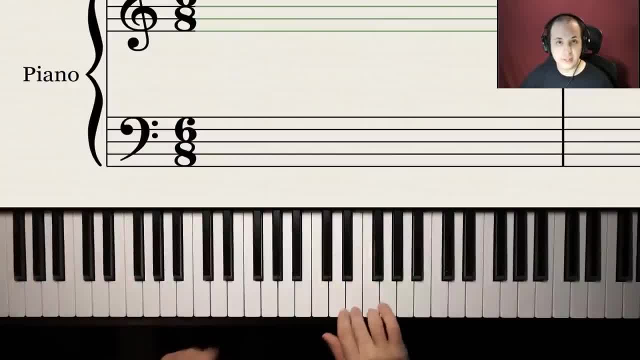 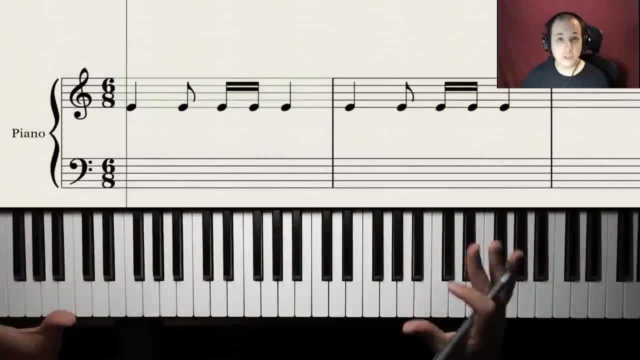 That you can have beats right And you play them smoothly, And that can be a form of rhythm. But just because it's a rhythm doesn't mean that it's exactly a beat. So to conclude, just going over some of the terms, 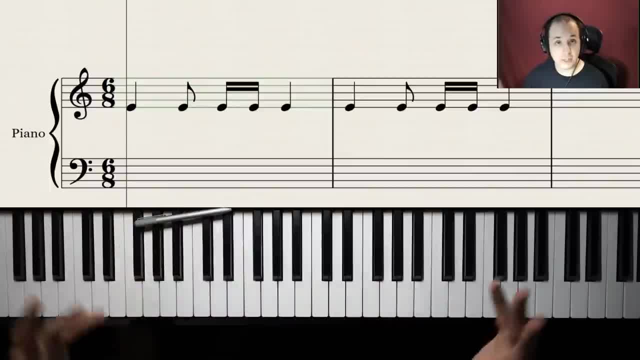 we talked about today. So the beat is the regular interval of sound, right, Like that. or let me play it on the piano. Beats are fit into these things we call Measures, right? You have a measure here and a measure here. 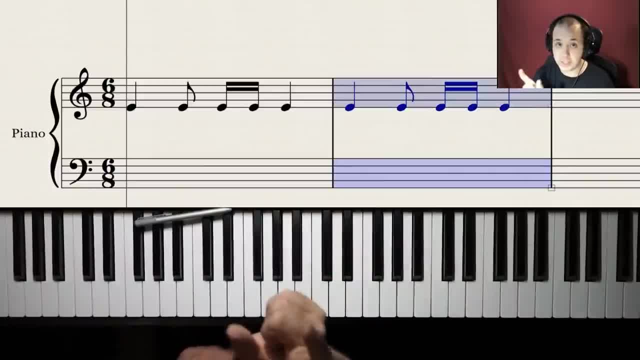 By the way, when you're counting beats in a measure, you're only counting one clef at a time. One of the mistakes a lot of people make is that they'll count both of them, But you're only counting one across because both clefs are actually being played simultaneously. 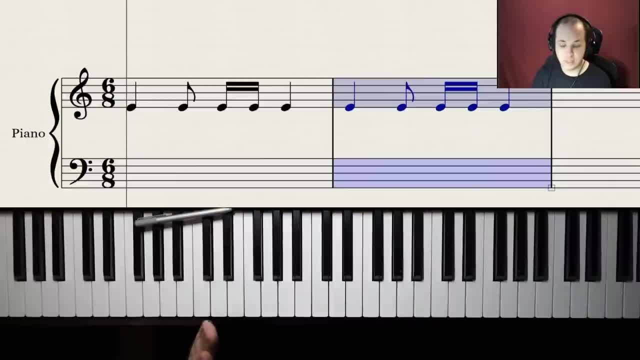 at the same time. So you're only gonna be counting the beats on one clef, And then obviously, the amount of beats up in the top clef should match the beats in the bottom clef. It doesn't have to have the same rhythm. 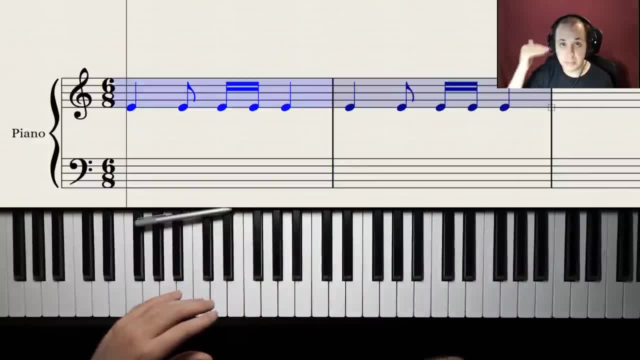 but it does have to like in 6-8. here we have to have six beats up top and six beats below. We're not gonna add those up to equal 12.. So that's one thing I just wanted to mention. 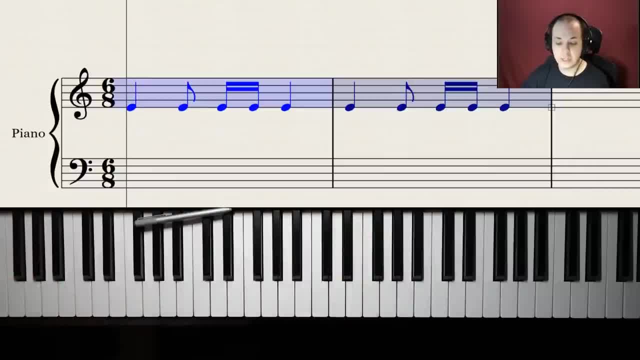 And then we also have our time signature tells us how many of the beats can fit in each of these measures. So that's how that fits together. And then, lastly, we have our rhythm, which a rhythm is just really a combination of note durations, which is another thing we talked about. 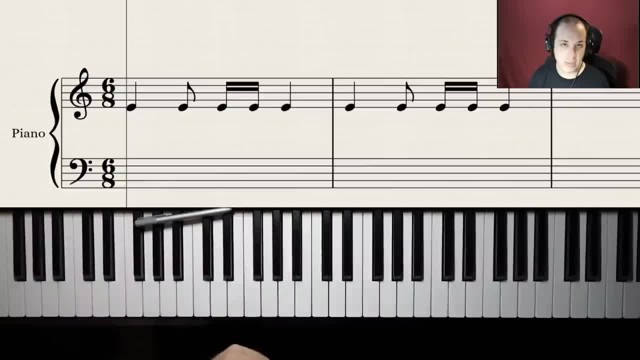 how long to play the notes. that forms a recognizable pattern to us and that is our rhythm that we have. So today's lesson was strictly just an introduction into rhythm, defining these terms, because I feel like these terms come up a lot. 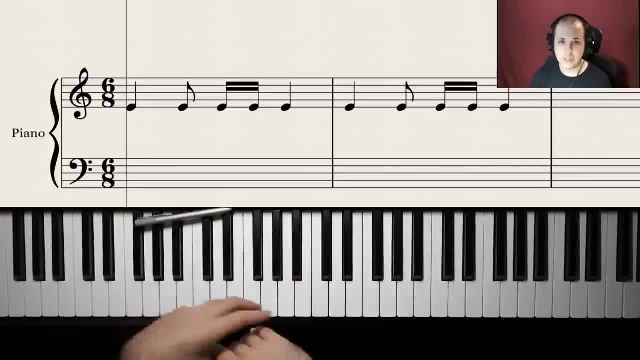 and people don't know exactly what they mean because they sound so similar- beats and rhythm and measures and time signatures and things like that. So the whole goal of this lesson was to fit them all together. So it's quiz time. 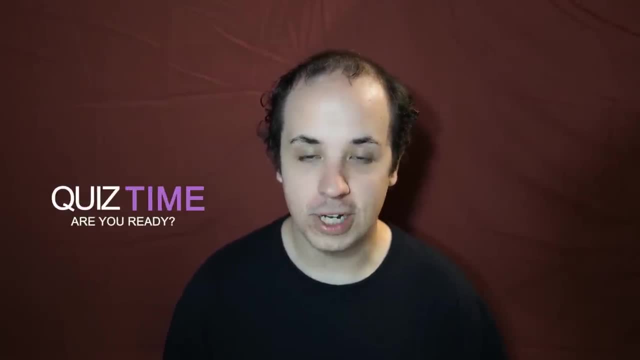 Are you ready? Just a couple of questions here for you today. Question one is: how would you do this? How would you define a beat? Question two is: what is a time signature and what does it do? what is it used for? 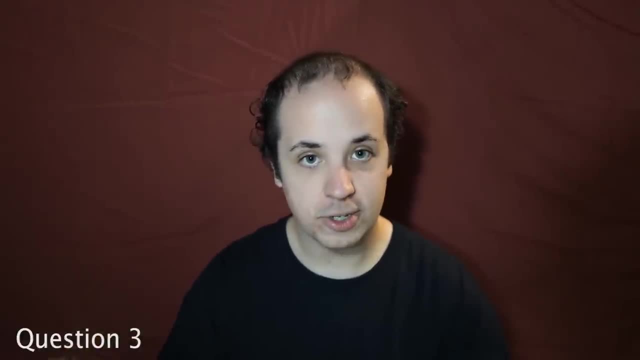 And then the third question is: the beats and the rhythms and all the stuff are organized into these little boxes, you know, divided by these vertical lines. What are the boxes called? So how'd you do If you got them all right? 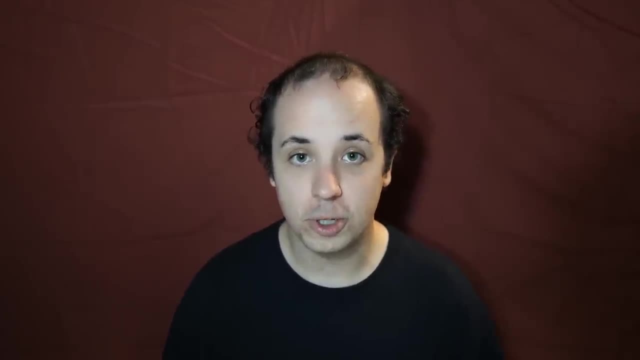 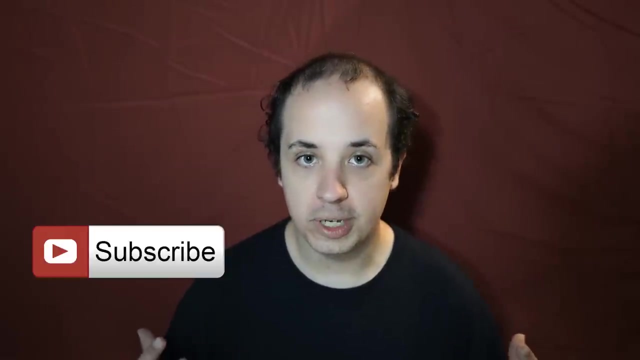 then you understand the lesson perfectly. If you didn't know the answer to some of the questions, then you should go back and watch the lesson again. And I want to tell you that you really should subscribe and become a part of our classroom, because there's new piano and music lessons. 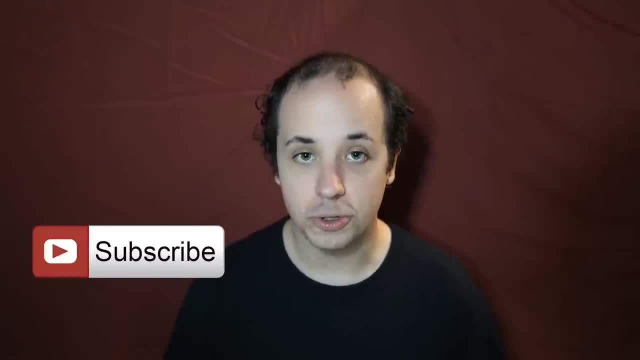 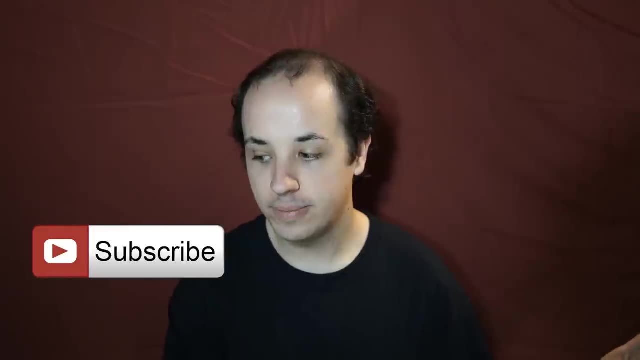 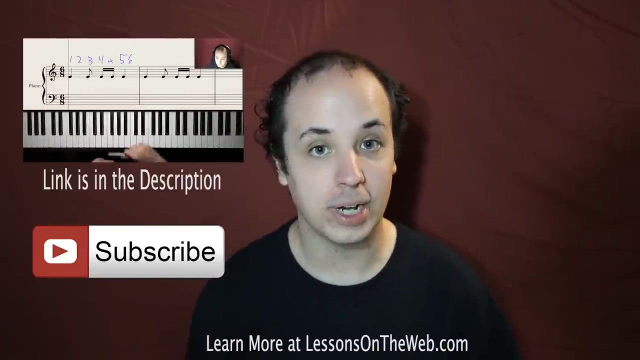 coming every Friday at 2 pm Eastern Standard Time. so you don't want to miss out on those great updates. And one last thing is you probably want to watch my playlist wherever it may be: playlist on rhythm itself, where we go through on how.